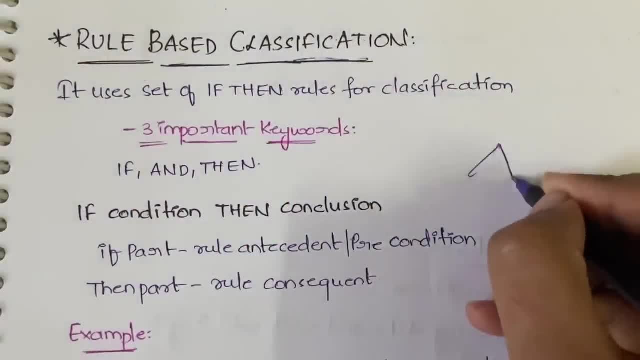 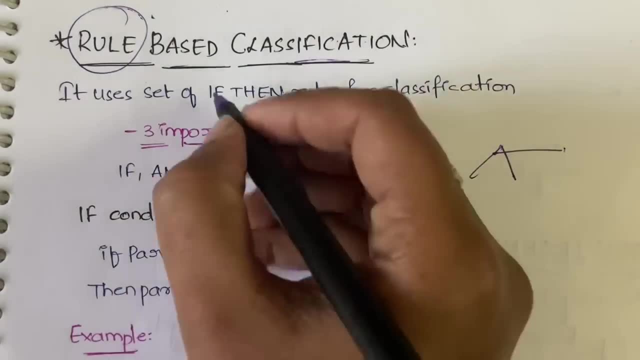 classification is nothing, but you'll be classifying the data into different number of categories based on the rules. Okay, that is called as a rule-based classification, and here the rules which you use are if-then rules- Okay. so here you will have three important keywords: if and 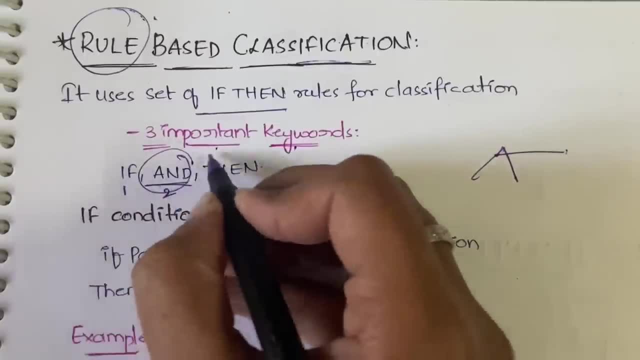 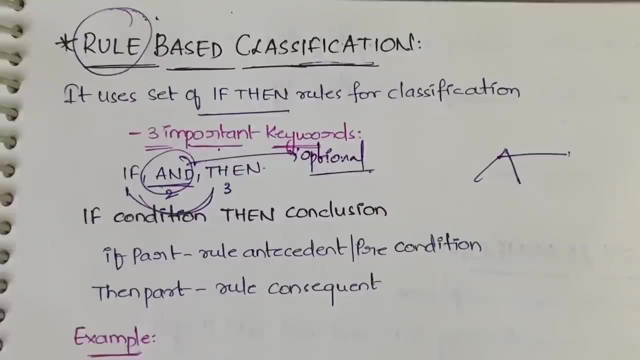 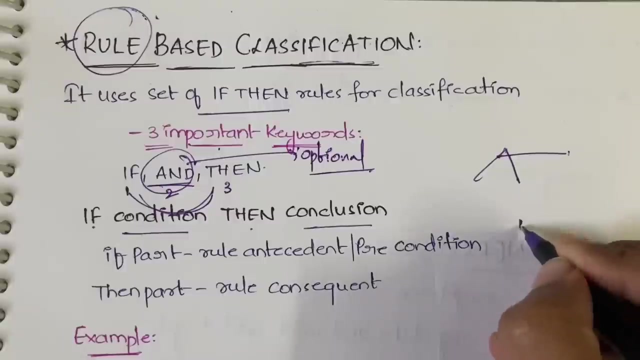 then Okay, so and is optional, and you don't find it in all the you know rules. but if and then will be in all the rules, Okay, I'll tell you with an example. So if the condition will be specified, then the conclusion will be specified. So, for example, if a is equal to true, then print high. 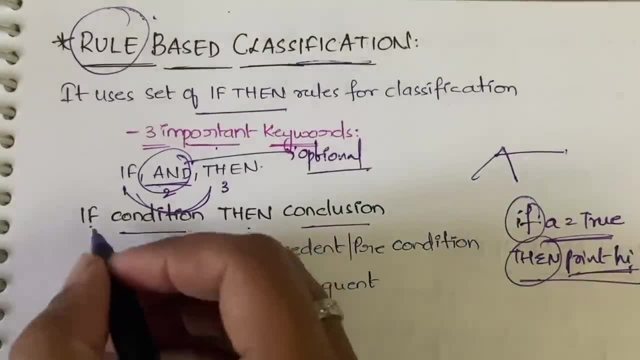 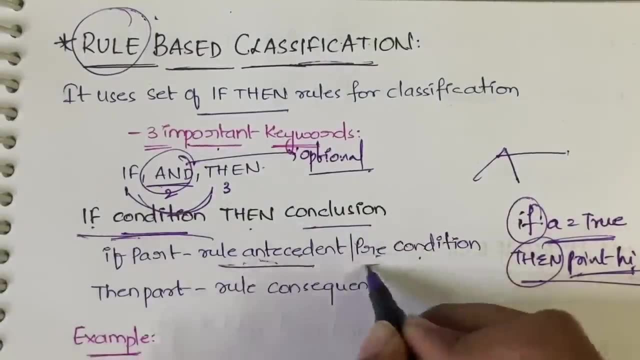 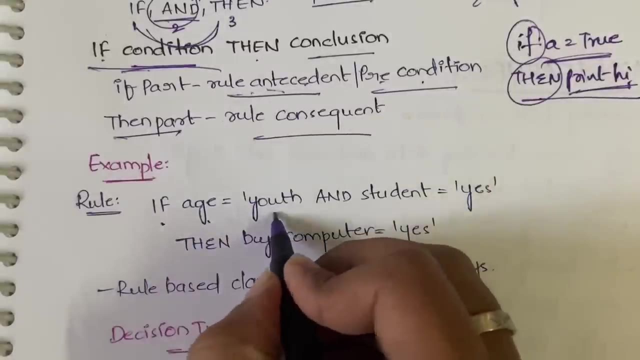 then a conclusion Got it. So and this: if part is called as the rule, antecedent or precondition, Okay, it is called as a rule, antecedent or precondition, The then part is called as the rule consequent. Next, for example, if age is equal to youth and student is equal to s, then by 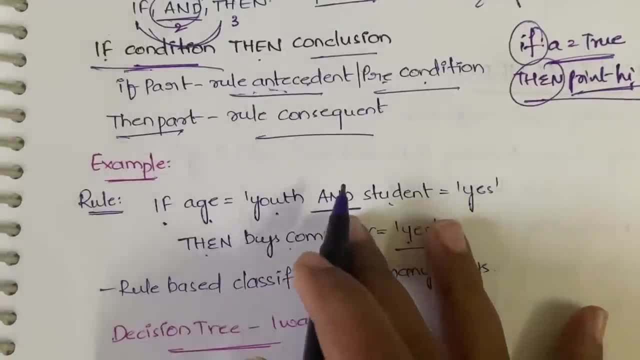 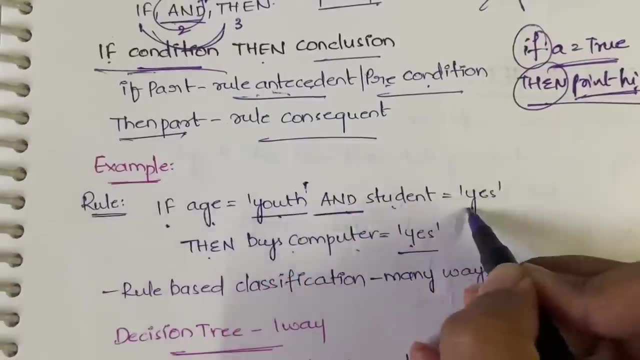 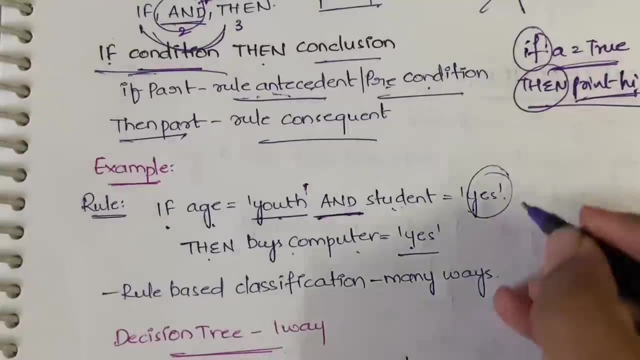 is equal to s. See, here we have, and Why? Because here we have two conditions. Condition number one is equal to youth and also the person has to be a student. Since we have two conditions we have, and If we have one more condition, you can write one more and and you can, you know, continue the condition. 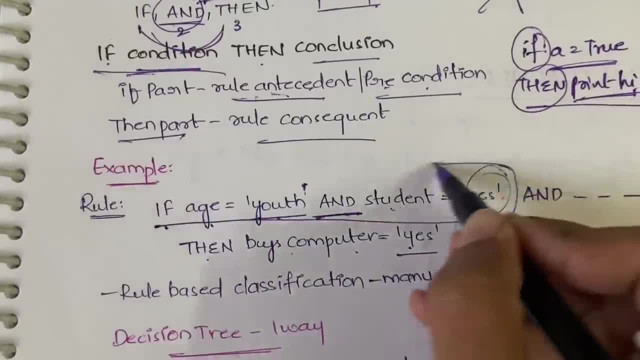 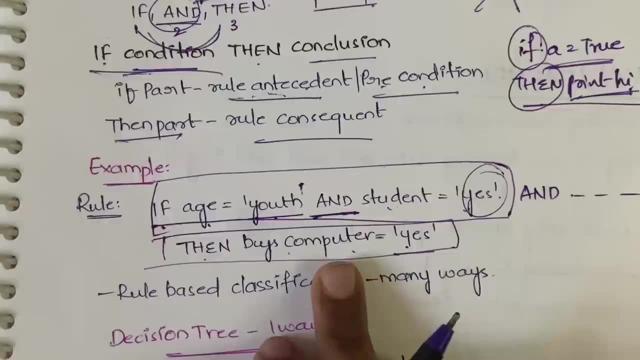 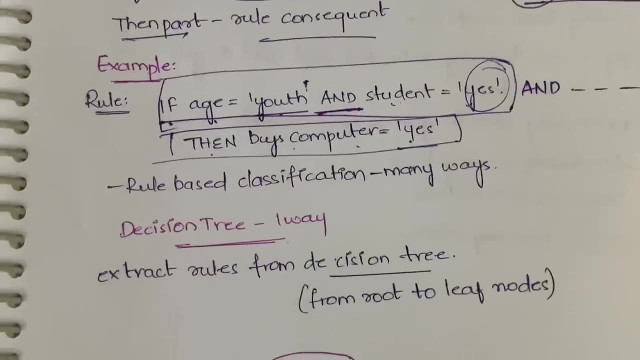 Got it. So now, here this up to, and all this part is called as the rule antecedent or the precondition. This then part is called as the rule consequent. Got it Now? so rule-based classification can be done in so many ways, but here, like we can do it with the help of decision tree, We can do it with. 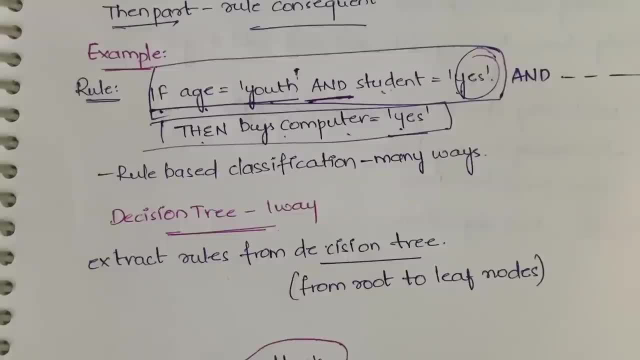 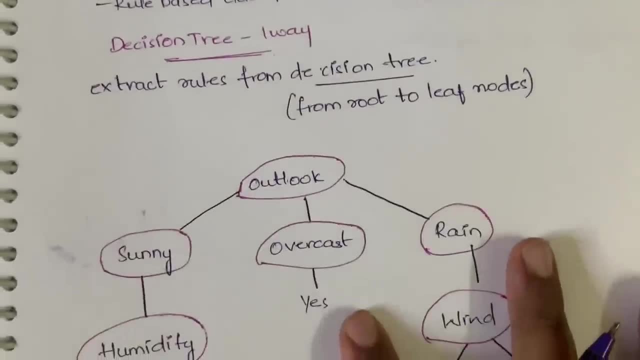 the help of different classifier algorithms and so on, but here in this video, let us see how we do it with the help of a decision tree. So, and with the decision tree, it is nothing, but you will have a decision tree like this. You will also you will be having a predefined tree like this and from this: 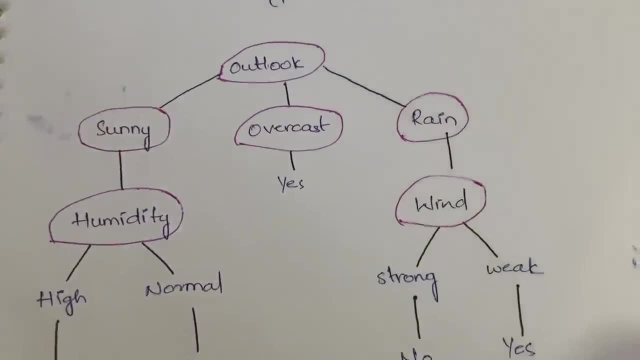 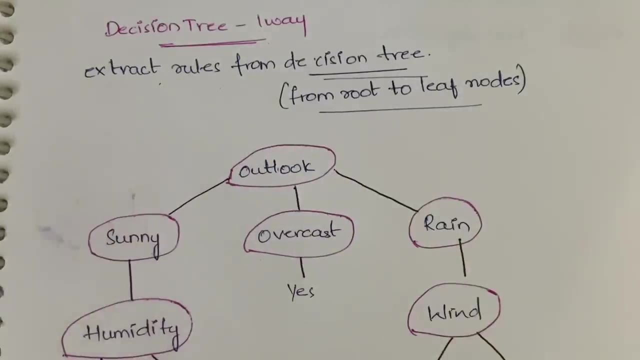 tree, you will be generating the rules. Okay, so you will be extracting the rules from the decision tree from root to leaf. I have written here Why? Because The rules should be extracted from the root to leaf, that is, you have to start from root and go to leaf. 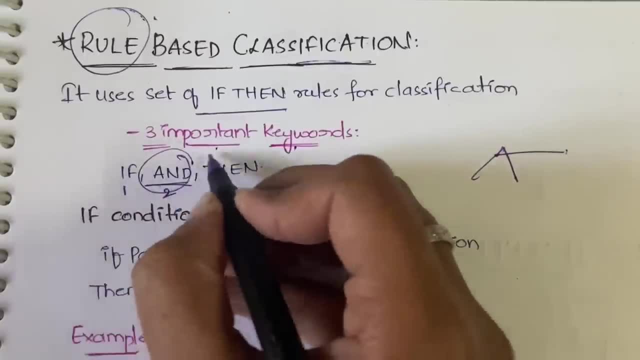 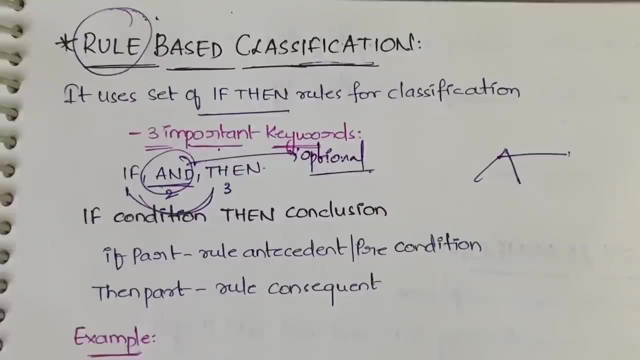 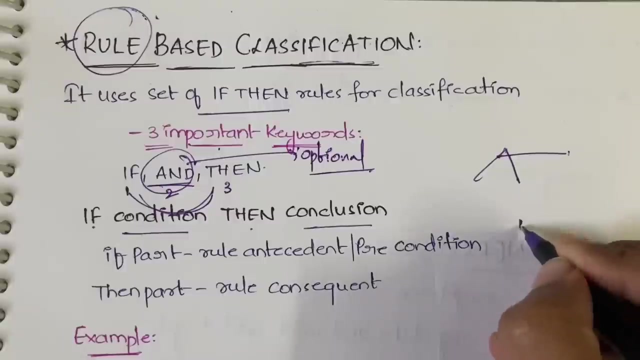 then Okay, so and is optional, and you don't find it in all the you know rules. but if and then will be in all the rules, Okay, I'll tell you with an example. So if the condition will be specified, then the conclusion will be specified. So, for example, if a is equal to true, then print high. 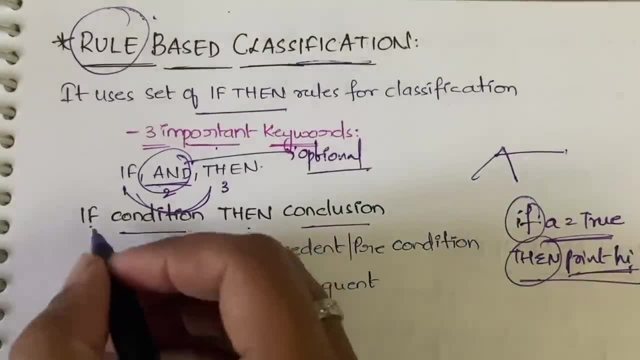 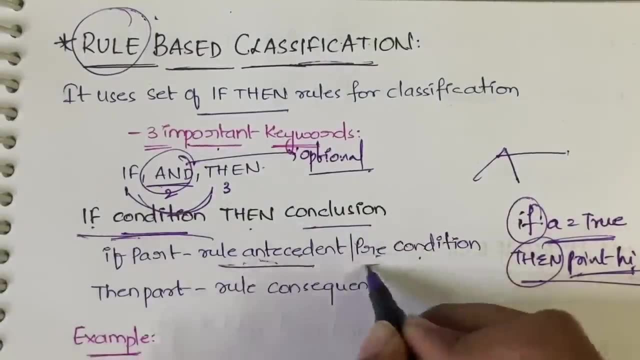 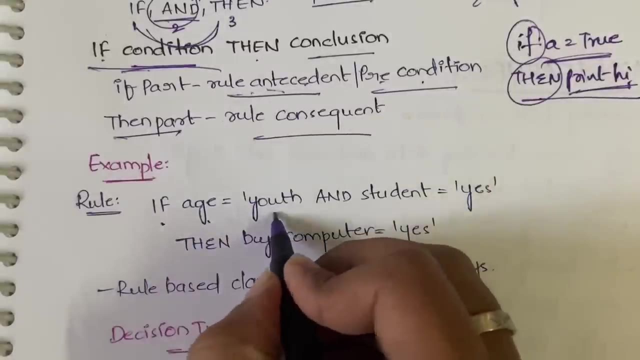 then a conclusion Got it. So and this: if part is called as the rule, antecedent or precondition, Okay, it is called as a rule, antecedent or precondition, The then part is called as the rule consequent. Next, for example, if age is equal to youth and student is equal to s, then by 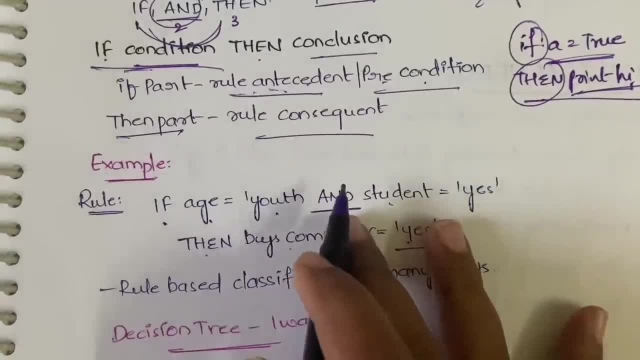 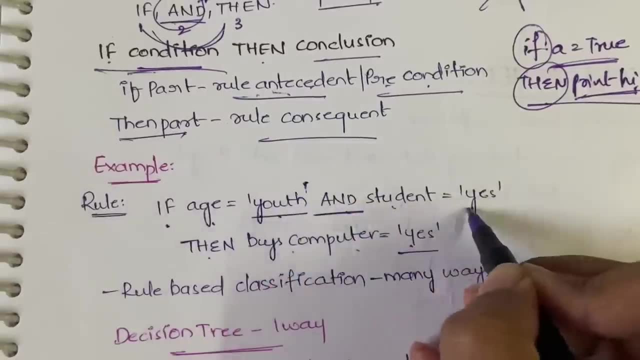 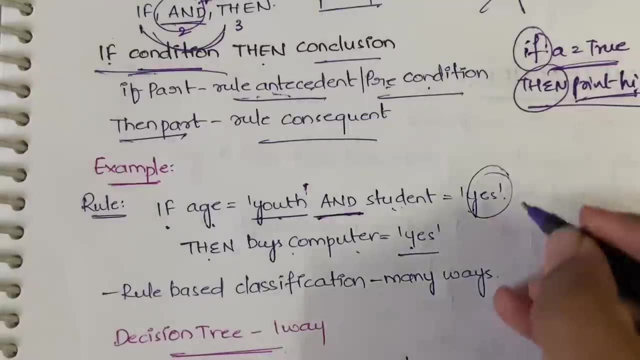 is equal to s? See, here we have, and Why? Because here we have two conditions: Condition number one to youth, and also the person has to be a student. Since we have two conditions we have, and If we have one more condition, you can write one more and and you can, you know, continue the condition. 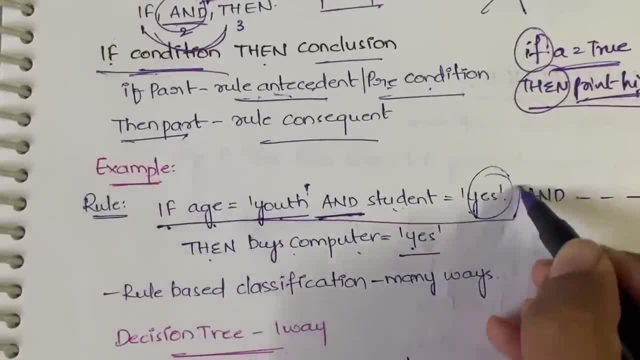 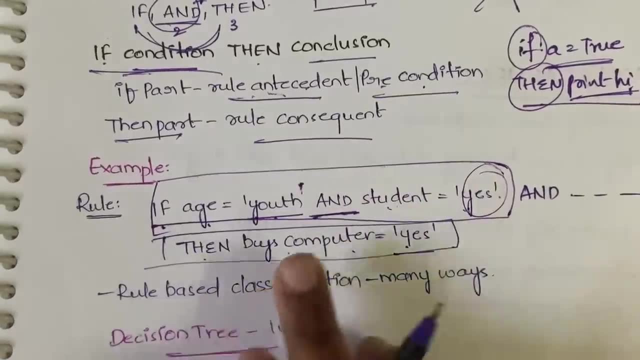 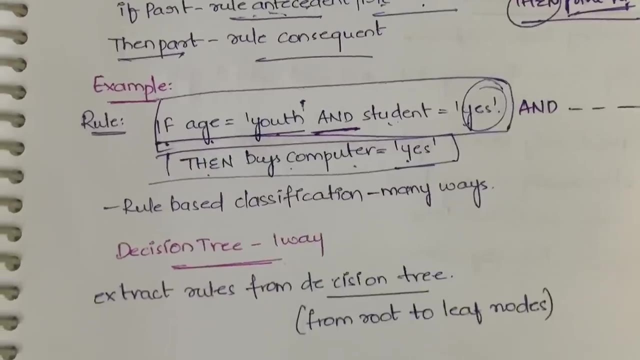 Got it. So now, here this up to, and all this part is called as the rule antecedent or the precondition. This then part is called as the rule consequent. Got it Now. so rule-based classification, so many ways, but here, like we can do it with the help of decision tree, We can do it with the help. 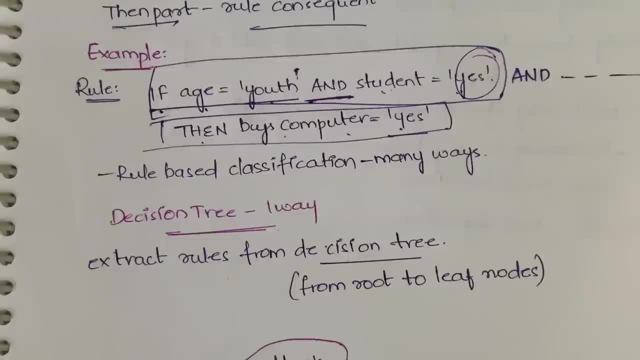 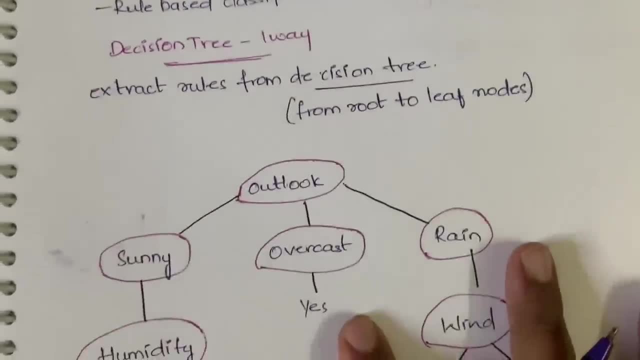 of different classifier algorithms and so on, But here in this video, let us see how we do it with the help of a decision tree. So, and with the decision tree, it is nothing, but you will have a decision tree like this. You will. also, you will be having a predefined tree like this and from 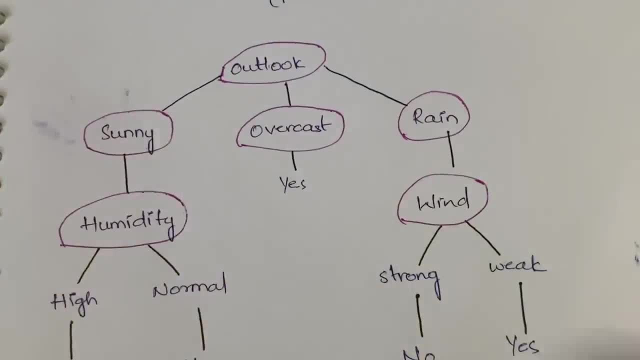 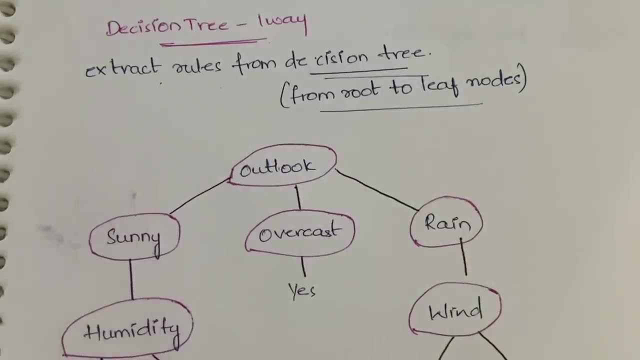 this tree, you will be generating the rules. Okay, So you will be extracting the rules from the decision tree From root to leaf. I have written here Why? Because The rules should be extracted from the root to leaf, That is, you have to start from root and go. 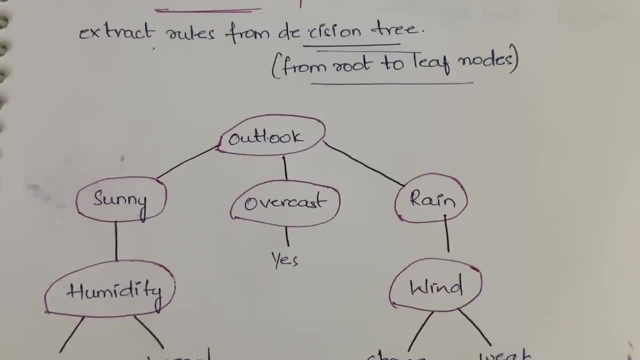 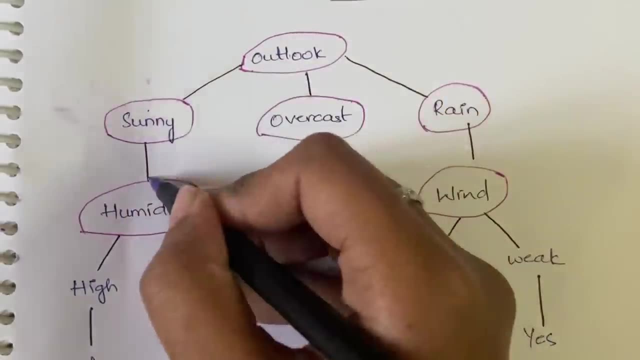 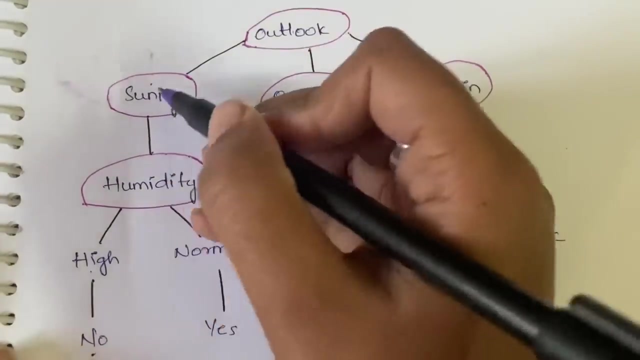 to leaf, That is, each and every node should be covered while you are extracting the rules, Got it? So here what rules you can extract. If outlook is equal to sunny and humidity is equal to high, then play is equal to no. Okay, Outlook is equal to sunny and humidity is equal to high, then play.